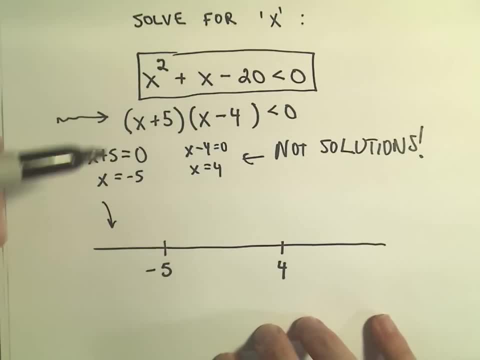 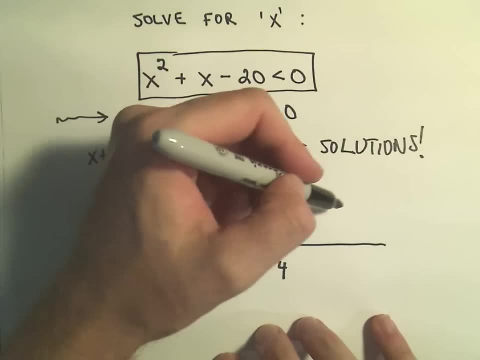 And then we're going to have to take a number smaller than negative 5, plug it into the inequality. We'll take a number in between negative 5 and 4, plug it into the inequality, see if it works. And we'll take a number bigger than 4, plug it into the inequality, see if it works. 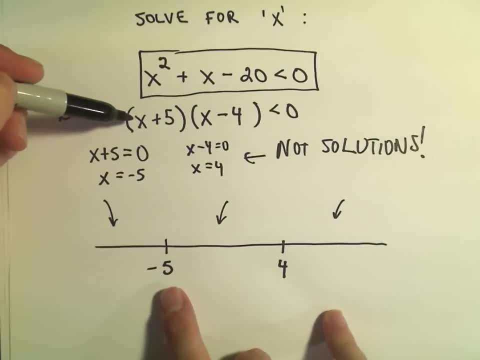 Notice if we plug negative 5 in, if we look at it in the factored form. notice if we plug negative 5 in, we would get 0 for the first factor. So the whole left side would turn into 0. And is 0 less than 0?? 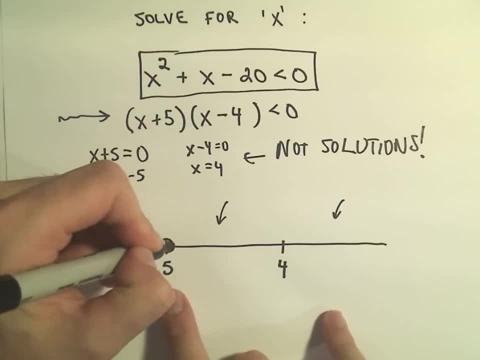 Well, it's equal to it, but it's not less than so. we don't use that, So I'm going to put an open circle to indicate that it doesn't work. Likewise, if you plug 4 in, we're going to get 0 out. 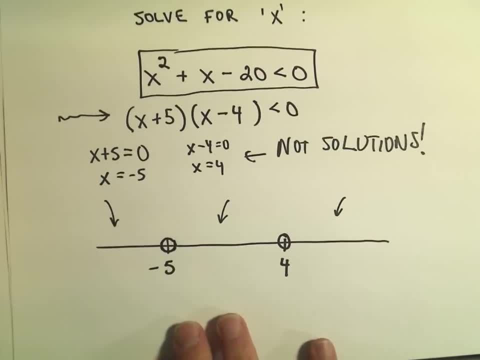 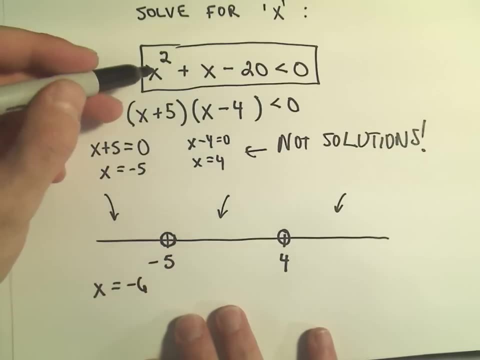 So that doesn't work, And now I just test points. I'll take a number less than negative 5. Maybe we can use x equals I don't know how. about negative 6?? So again, I'm going to plug it back into the inequality. 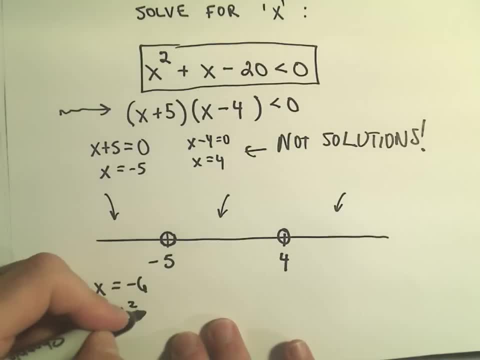 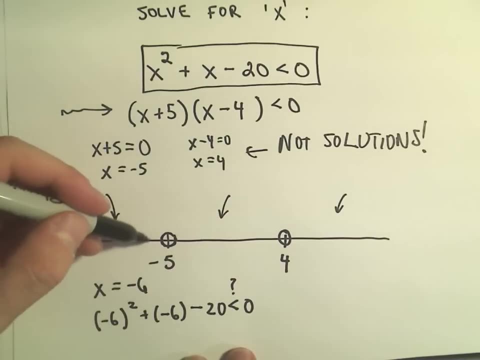 So I'm kind of asking myself: is negative 6 squared plus negative 6 minus 20,? is that less than 0?? If so, I'm going to shade everything to the left, And if not, it says: it turns out that nothing smaller than negative 5 will satisfy the inequality. 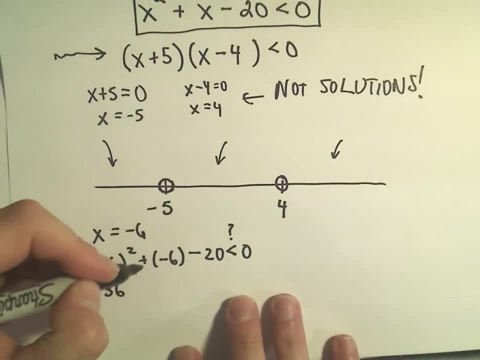 Okay, so negative 6 times negative 6 is 36, plus a negative 6 is just minus 6 minus 20.. And I'm thinking: is that less than 0?? Well, notice on the left, we would get 36 minus 6,, which is 30, minus 20 is going to be 10.. 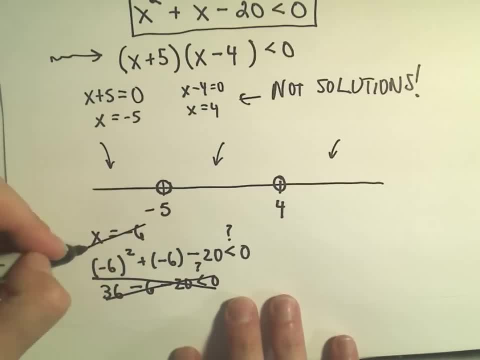 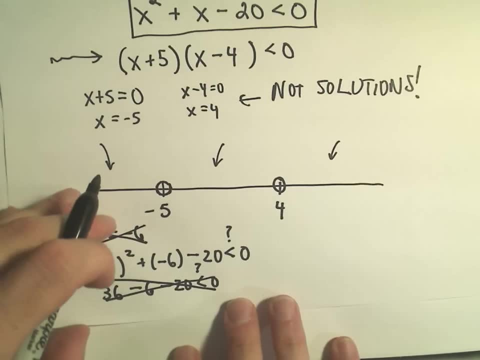 10 is not less than 0. So that means negative 6 didn't work. So it means any number smaller than negative 5 also does not work. Okay, next we'll ask ourselves: we'll take a number between negative 5 and 0. 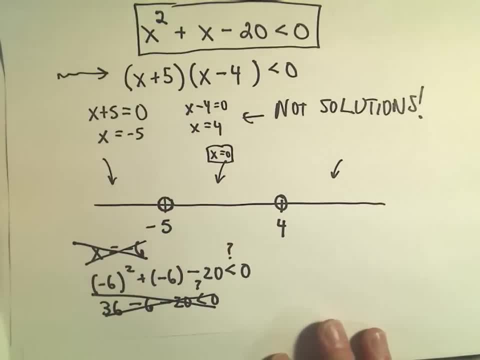 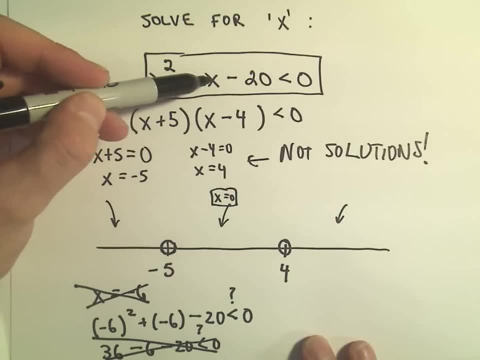 I'm going to use any number at random. I'm going to use 0, just because that will make the arithmetic easy. And notice, if we plug 0 in, we'll get 0.. 0 squared plus 0, which, well, that just leaves us with 0.. 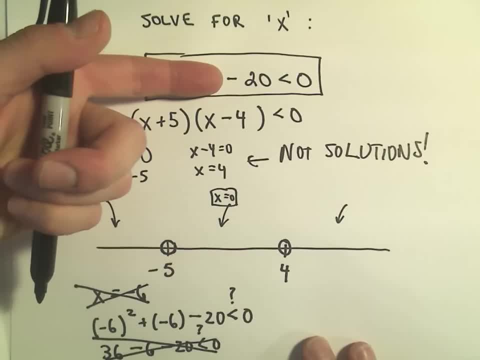 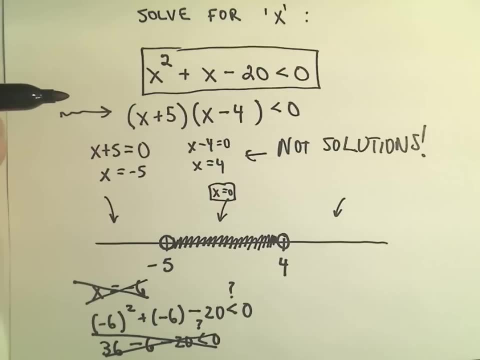 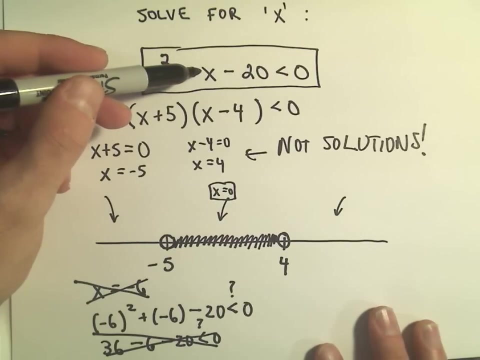 And then we would be left with negative 20.. Negative 20 is less than 0, so that tells me everything in the middle works. And now we take any number bigger than 4.. Maybe I'll take a million. Well, notice, if you take a million and square it and add a million, that's going to be a big positive number.